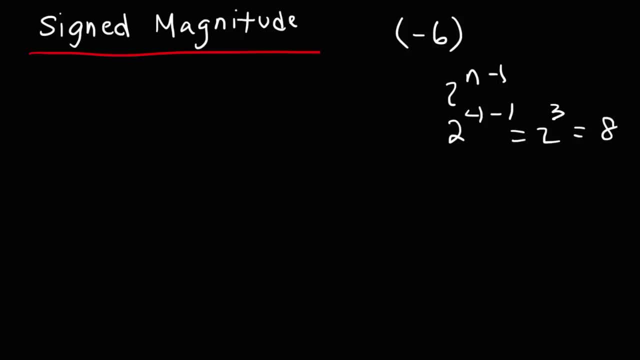 to the four minus one, which is two to the three, and that's eight. So this is going to be eight, four, two and one. So first let's express the sine magnitude method, And we're going to use a four-bit binary to do so. 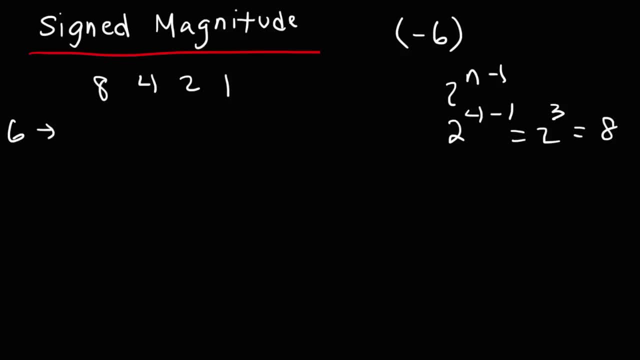 So we're going to put a one in the column under four and two and we're going to put a zero everywhere else. So that would be positive. six In sine magnitude. the first three numbers corresponds to the magnitude of the number six. The last number, zero. this corresponds to the 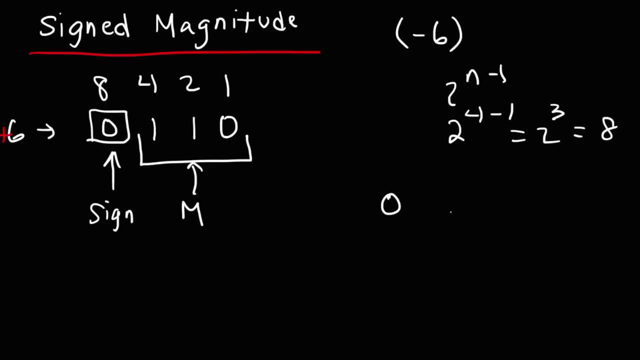 sine. So if the last number is zero, that means we're dealing with a positive number. If it's one, that means we're dealing with a negative number. So to express negative six, we just need to replace this with a one, So using the sine magnitude method. 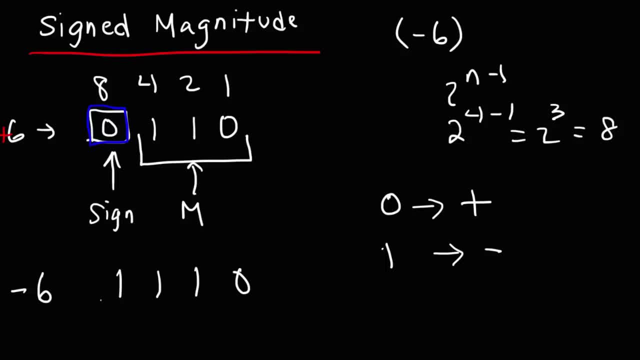 negative six is going to be one one, one zero, And that will be the answer. Now let's work on some other examples. Using the sine magnitude method, let's express the following numbers: So if the last number is zero, that means we're dealing with a positive number. 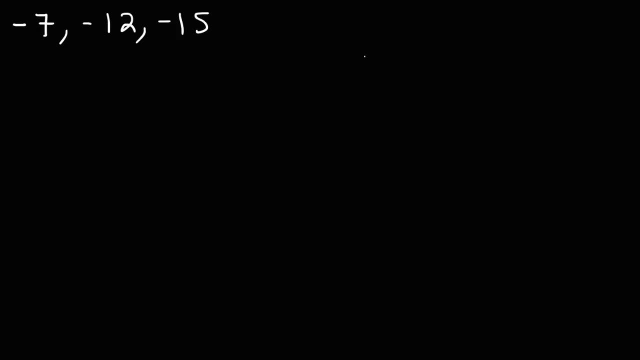 We're going to use the following negative numbers in binary And we're going to use a five-bit binary system. So two to the n minus one, that's going to be two to the five minus one, which is two to the four, and that's 16.. So this is going to be 16, eight, four, two and one. So let's start with. 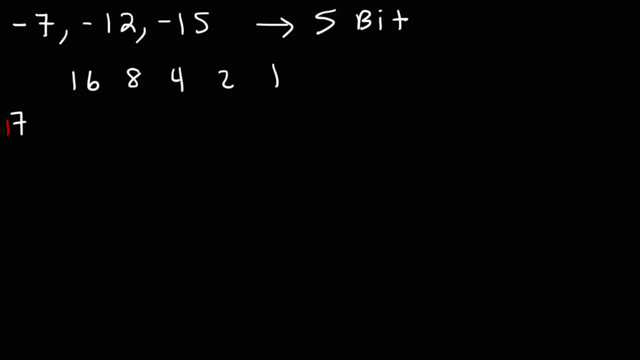 positive seven. Because this is positive, the first one is going to be zero. Seven is four plus two plus one, So we're going to put a one under those numbers, So that number corresponds to seven. To get negative seven, all we need to do is replace this zero with a one. Remember that first number. 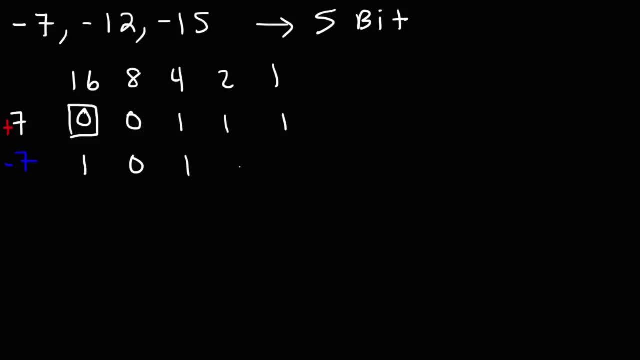 indicates a sine. Everything else is going to be the same. So using the sine magnitude method, negative seven would correspond to this five-bit binary number. Now let's try a negative 12.. So first let's find the number for 12.. So the first number is going to be a zero and 12 is simply eight plus four. So we're going to 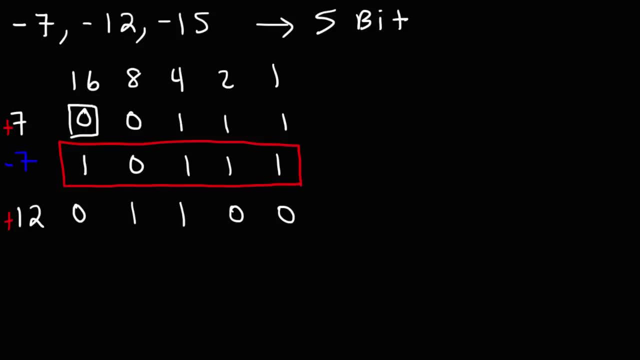 put a one under those two numbers, So that's the binary equivalent of 12.. So now let's find a negative 12.. So we're just going to replace this with a one, So it's going to be a negative 12.. 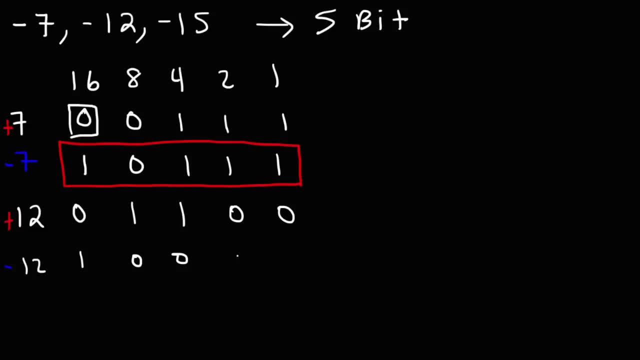 It's going to be one zero zero. I mean one, one, one zero zero. We're just changing that number into a one, And so that's how we can represent negative 12, using sine magnitude. For the last one, negative 15,, let's start with positive 15.. So the first number is going to be: 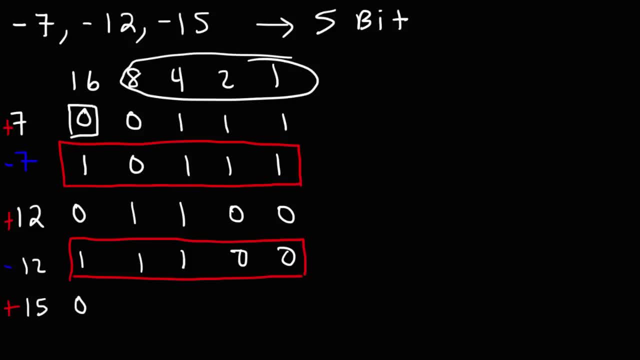 zero 15 is the sum of all four of these numbers. Eight plus four plus two plus one is 15.. So we're going to put a one for all four of them. So to express negative 15, change the sign to negative. 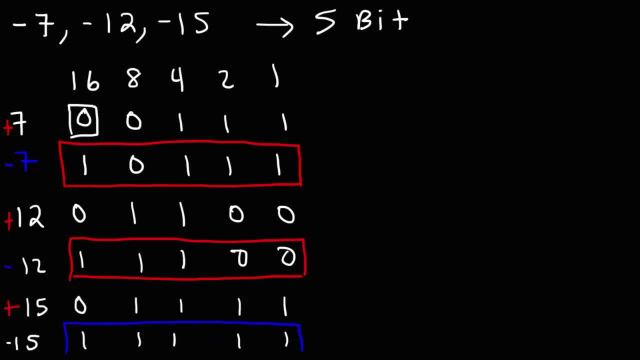 So this would be the five-bit binary number that will correspond to negative 15.. So this method of representing negative numbers, that is, the sine magnitude method, is very easy for people to understand. It's very user-friendly. However, it doesn't work very well for computers. 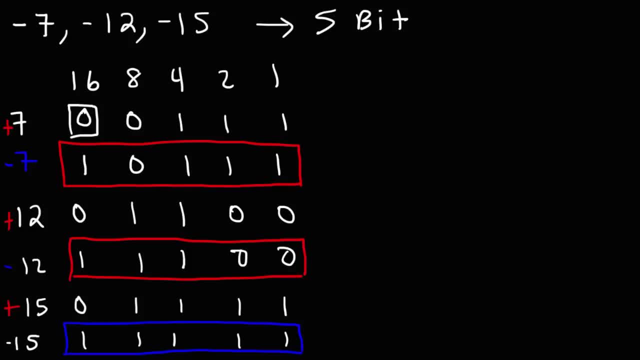 especially when computers need to perform operations Such as addition or subtraction, For instance. let's say, if we want to add seven and negative seven, we should get zero. So let's add these two binary numbers: zero, zero, one, one, one. 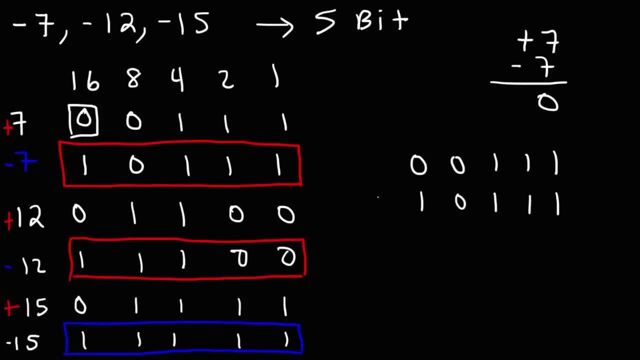 and one one, one zero one. So one plus one, that would be two, but we can't really write two, So we'll just put zero carry over the one. Right here would be zero carry over the one, but we have another one plus this zero, which? 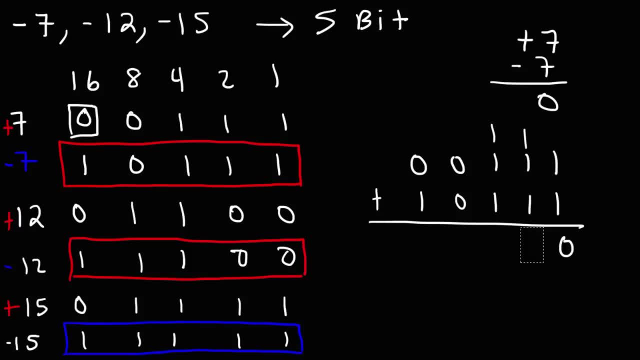 will turn this into a one. So this right here would put a zero and a one, carry over, but the zero part plus this one will give us another one, And then we have one plus zero, which is one, and zero plus one, which is one. 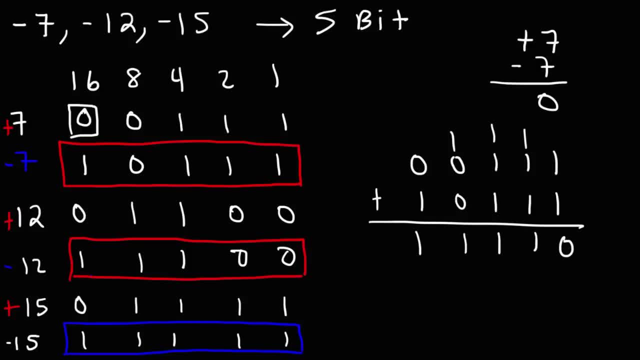 Right here would be one and zero, plus one, which is one, And this is one, two, four, eight, 16.. So we're adding sixteen, eight, four and two, So the result that we'll get is not zero. as you can see, This would be 30, and that. 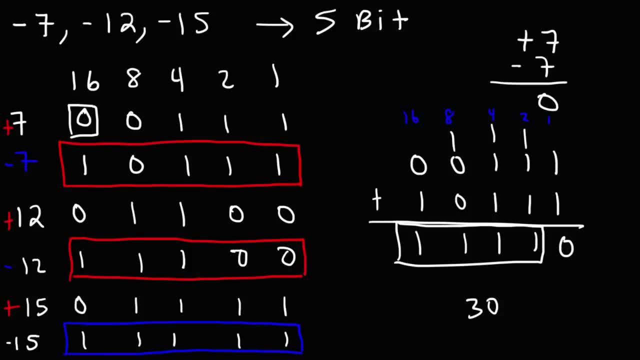 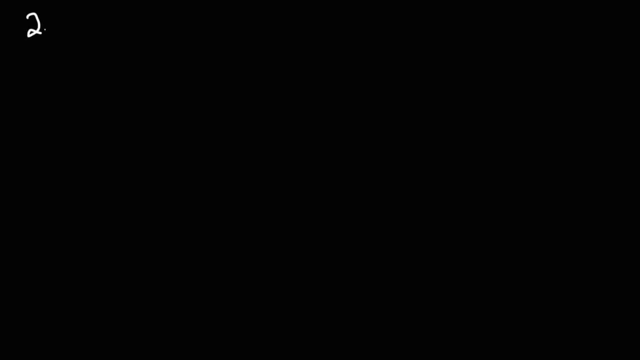 can't be right. So, as you can see, when expressing negative numbers using the sign and magnitude method, It's not very helpful if we need to perform operations such as addition or subtraction. So now let's talk about expressing negative numbers using the 2's complement method. 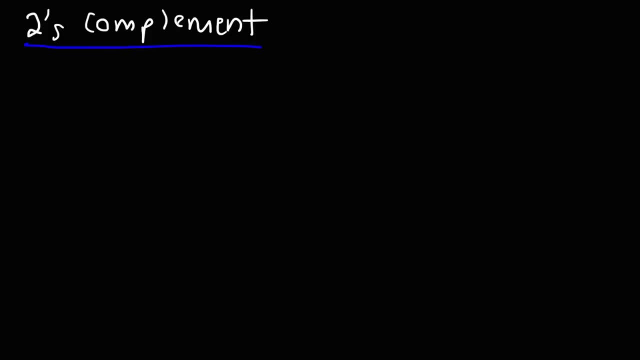 And we're going to see why this works out so well. So let's start with 7.. So 7 is 0, 1, 1, 1.. Now what we need to do is find the 1's complement first. 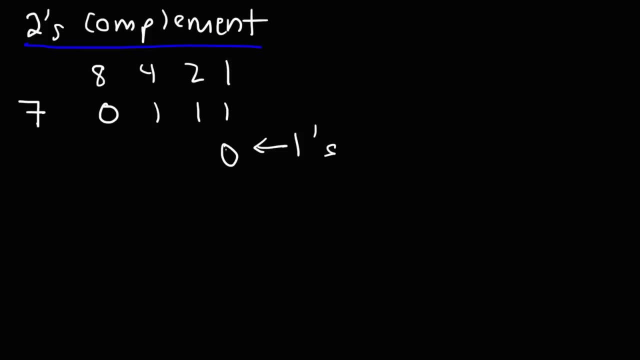 So we're just going to: every 1 that we see we're going to replace it with a 0. And every 0 that we see we're going to replace it with 1.. Now our next step is to add 1.. 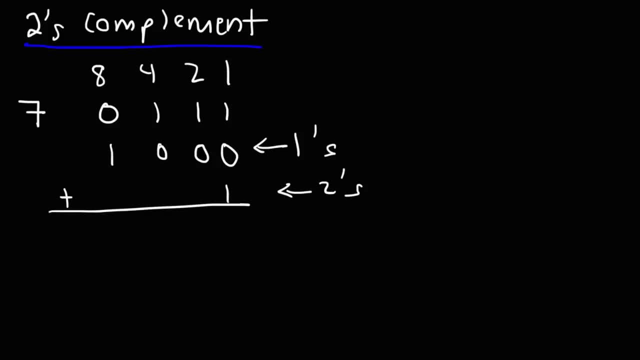 That will give us the 2's complement. 0 plus 1 is 1.. And then we could just bring down everything else. So negative 1 is 1. And negative 7 would correspond to the number that we see here. 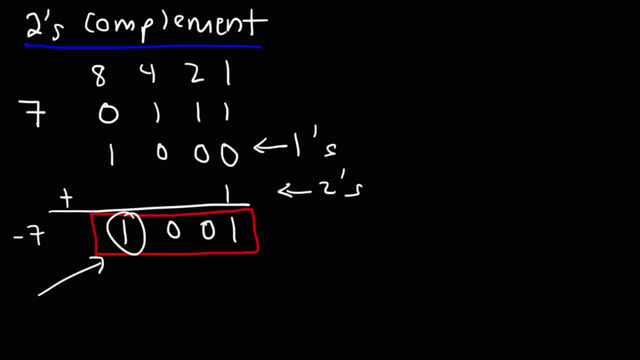 Now keep in mind: the first 1 that you see indicates a negative value. Now how can we quickly check to see if this is indeed negative 7? Because the binary equivalent looks like 8 plus 1, which is 9.. But here's how you can check to see if it's negative 7.. 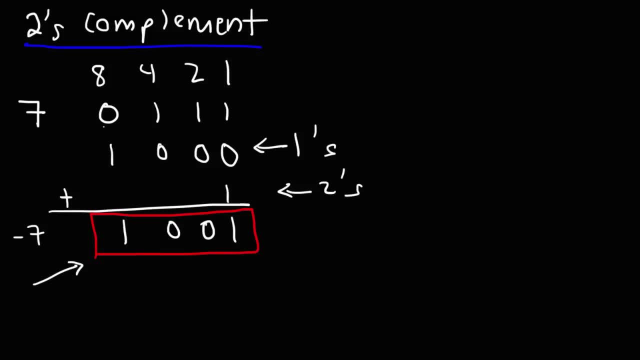 Remember, Negative 1 is associated with a negative sign. So if you make this negative 8, this becomes negative 8 plus 0 plus 0 plus 1, which gives us negative 7.. So that works. So that's how we can represent a negative number. 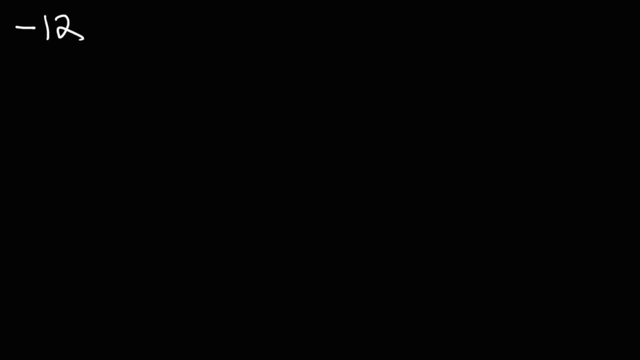 Let's try another example. So go ahead and represent negative 12 as a binary number using the 2's complement. So first We're going to use a 5-bit system, So 16, 8,, 4,, 2, 1.. 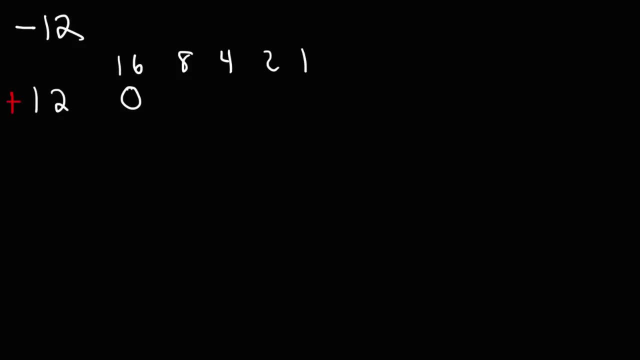 So the 0 would indicate that this is going to be a positive number, just like before. So that's why we're using the 5-bit binary system instead of a 4-bit, Because we need the 8 to make 12.. 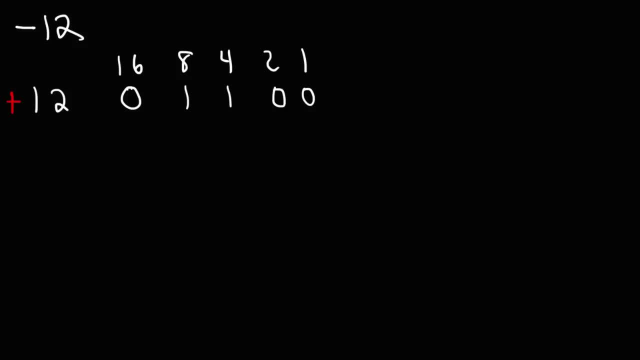 8 plus 4 is 12.. So 12 would be 0, 1, 1, 0, 0.. Now Let's find the complement of this number. So replace 0 with 1 and replace 1 with 0.. 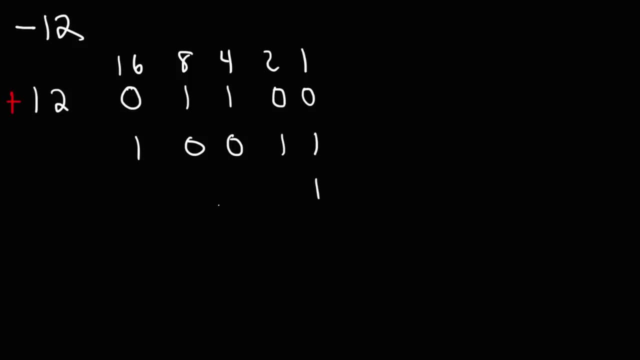 Next Add 1.. So 1 plus 1 is going to be 0, carry over the 1.. 1 plus 1 is 0, carry over the 1.. Let me just separate these numbers from what we have below. 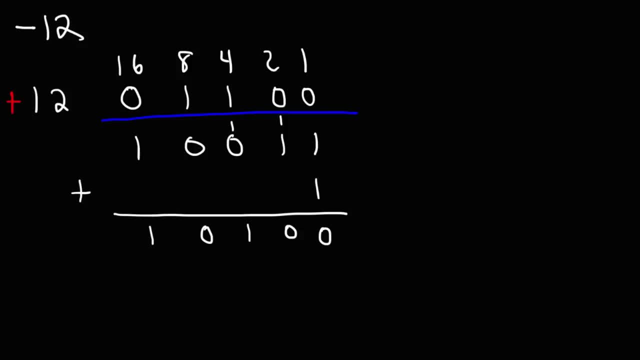 1 plus 0 is 1.. And then we can just bring down the other numbers. So negative 12 is 1, 0, 1, 0, 0.. So keep in mind, the first number is to tell us that it's a negative number. 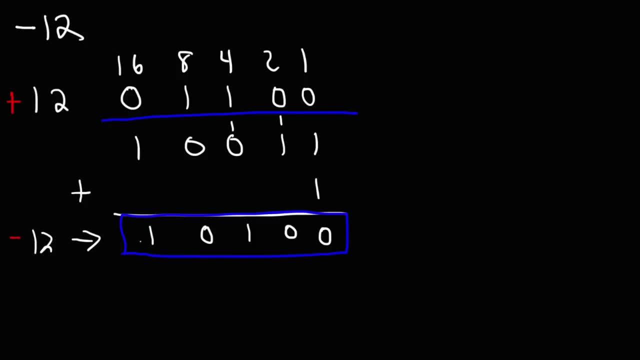 So now let's check our work. So we have a 16 here and a negative value, So that's going to be negative 16.. We have a 0 in the 8 column, so we're not going to add anything. We have a 1 in the 4 column, so we're going to add a 4.. 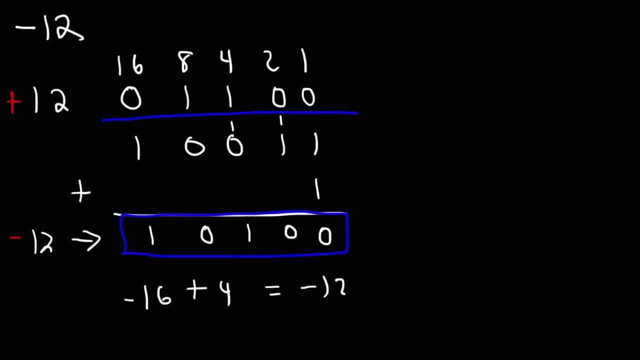 And here we have nothing. So it becomes negative 16 plus 4.. And that checks out That is negative 12.. So that is negative 12 as a binary number using the 2's complement method. So now let's talk about how we could subtract two binary numbers. 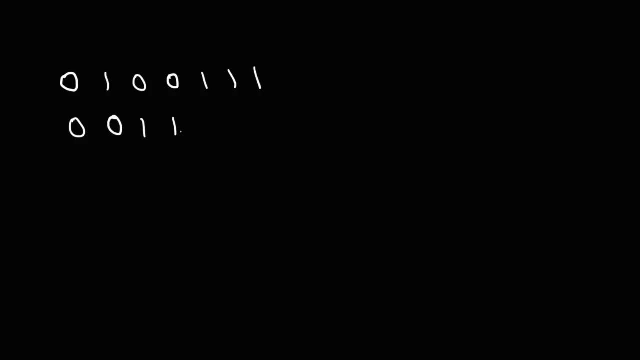 Okay, So We're going to go over two methods. The first one involves straightforward subtraction And the second one involves the 2's complement. So let's do straightforward subtraction: 1 minus 1 is 0.. 1 minus 0 is 1.. 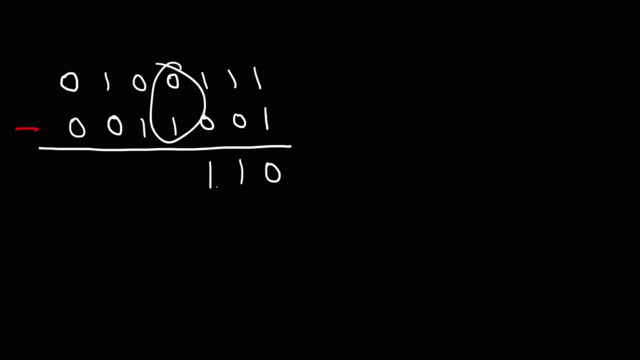 Now 0 minus 1, if we do that, that's going to be negative 1.. And putting a negative 1 here just doesn't look right. So let's not do that. What we need to do, What we need to do, is borrow something from this 1.. 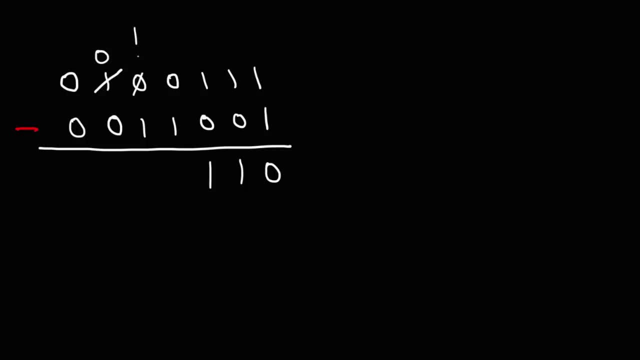 If we borrow a 1, this becomes 0. And we get two 1's here. Now we're going to have a lot of 1's here, So that just doesn't look right. I mean, you could do it this way. 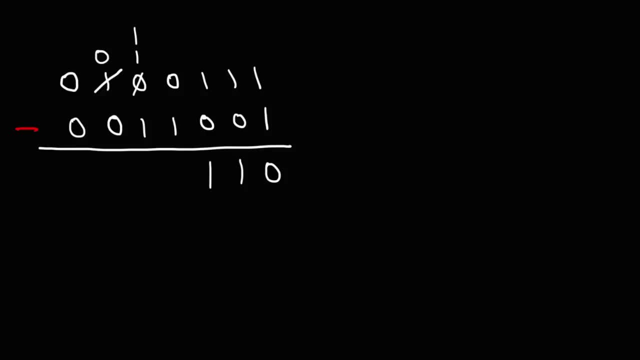 It works, But the decimal equivalent of two 1's is 2.. So I like to represent this as 2.. That's just my unconventional method of subtracting binary numbers. Now we need to borrow a 1 from this 2.. 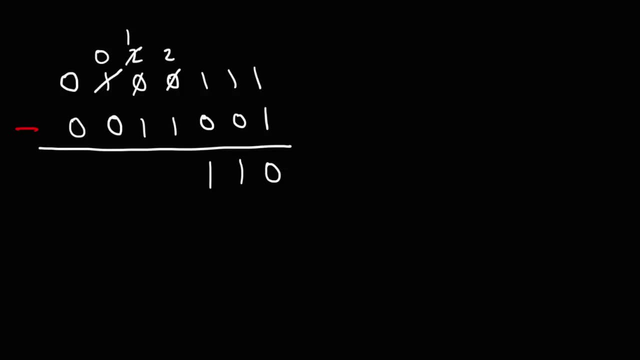 Okay, And so this is going to become a 2.. 2 minus 1 is 1.. 1 minus 1 is 0.. And then 0 minus 0 is just 0.. So now let's see if this actually works. 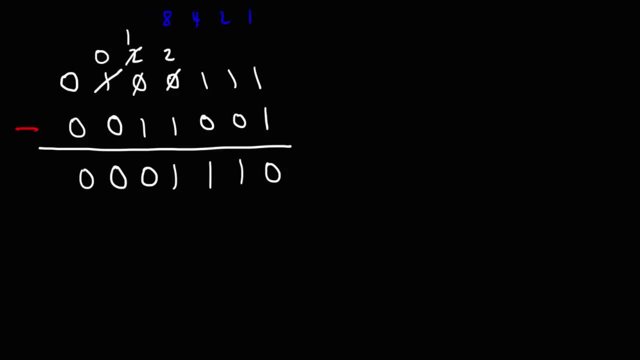 So this is 1, 2,, 4,, 8,, 16,, 32,, 64.. So now let's convert these numbers into decimal numbers. Okay, So we're going to have a 1 here. So originally we had a 1 here. 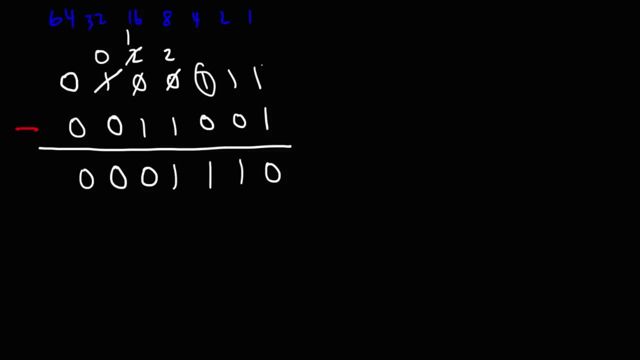 The decimal value for that is 32.. Plus 4, that's 36.. Plus 2, 38.. Plus 1,: 39. So the original number at the top was 39. And then we have a minus sign. This is 16 plus 8, that's 24, plus 1, that's 25.. 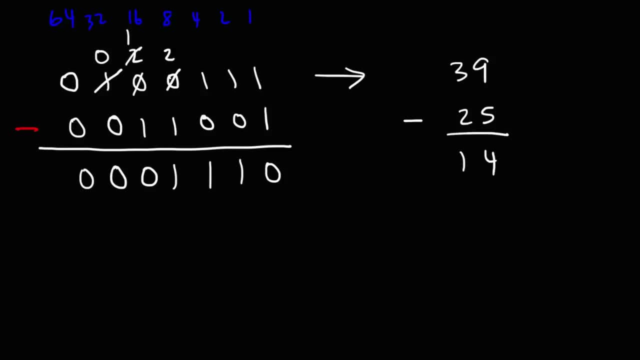 So 39 minus 25,, that's 14.. Now let's see if this number actually works, If this number actually represents 14.. So this is 8, 4, that's 12, plus 2, that is 14.. 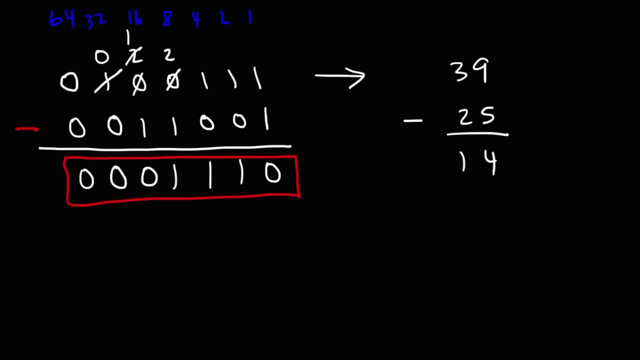 So this technique works. It's a very simple way of subtracting two numbers. Now let's use the 2's complement method. In this example, we subtracted two positive numbers. We had positive 39 minus positive 25.. Now, when using the 2's complement method, if you need to do subtraction what you want. 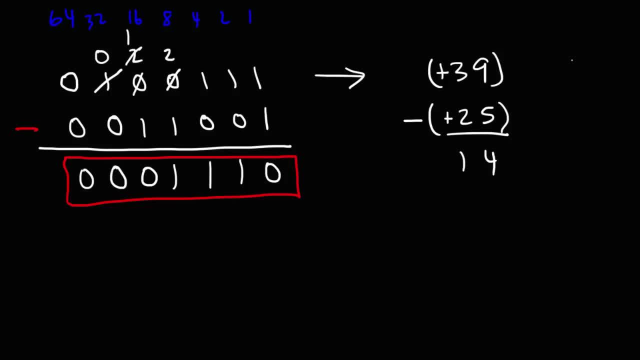 to do is basically add a negative number, So this is still going to be positive 39. I'm just going to write 39 to represent that, And then it's going to be plus negative 25.. We're still going to get 14.. 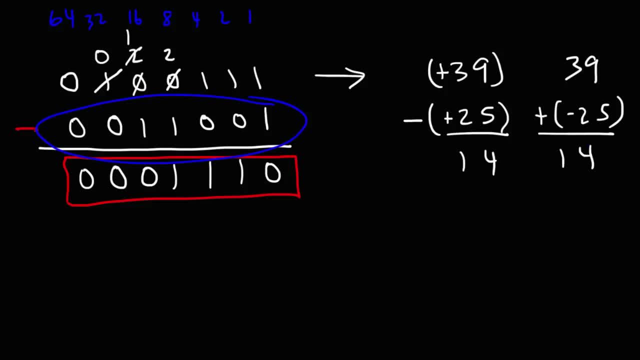 But instead of having a positive 25 value here, we're going to have a negative 25.. So I'm going to rewrite the 39 value. I'm going to write 49 as a primary number. So that's what we have in this row. 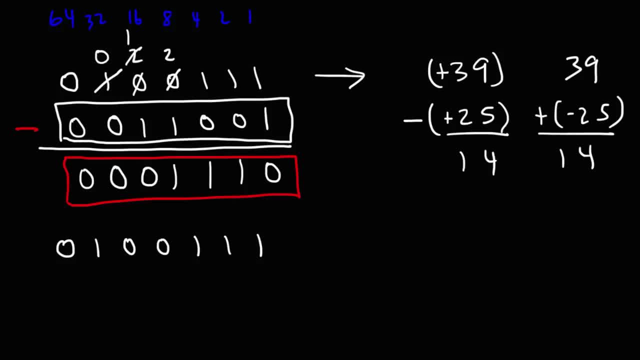 Now I'm going to change this part which is positive 25, into negative 25, using the 2's complement method. So first let's rewrite it, Now let's find the 1's complement of that number, So replace 1 with 0. 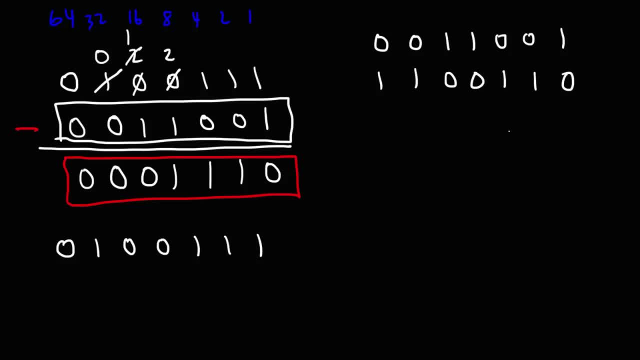 And then replace 0 with 1.. Our next step is to add one, So this is 1 1 1 0, 0 1, 1.. So this number should represent negative 25.. And let's just check it to make sure that it does So. 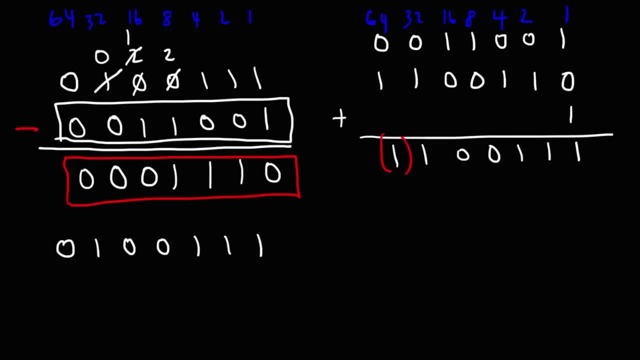 keep in mind. the first one represents a negative value, So that's going to be negative 64. So we have negative 64 plus 32. This corresponds to a 4. So that's plus 4 plus 2 plus 1.. Negative 64 plus 32 plus 4 plus 2 plus 1. So that is. 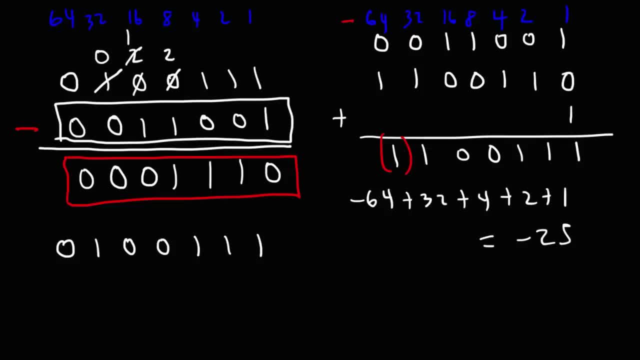 indeed negative, 25.. So now I'm going to take this binary number and put it beneath this one, So that's 1 1 0 0, 1 1, 1.. And now we're not going to subtract, but we're going to add. So 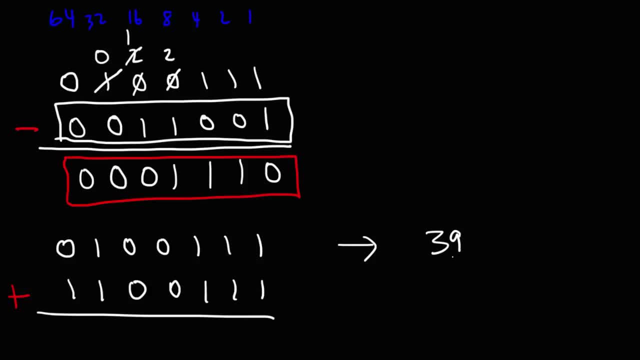 remember, the top number is positive 39. The bottom number is negative 25.. And we're adding, which is a nice way to do subtraction. So 1 plus 1, that's going to be 0. Carry over the 1.. Now this part here: 1 plus 1, that is 0. Carry over the 1.. But 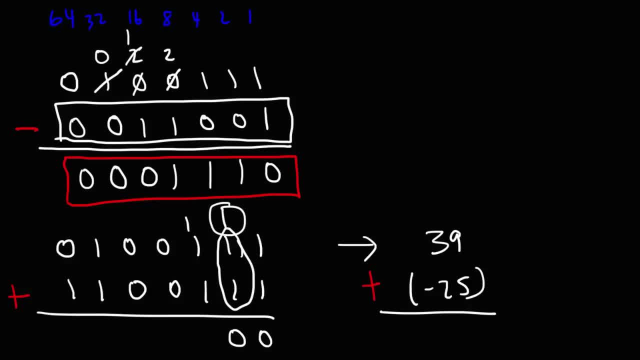 when you add this 1 and this 0,, that becomes a 1.. Now we're going to do the same thing here: 1 plus 1 is 0.. Carry over the 1.. And then 1 plus this 0 is 1.. 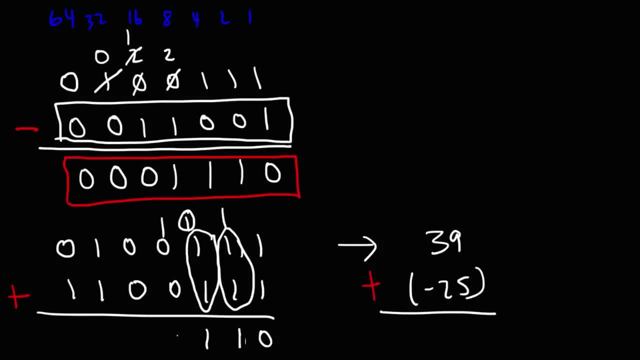 Now we have 1 plus 0 plus 0, which is 1.. 0 plus 0 is 0.. 1 plus 1 is 0.. Carry over the 1.. 1 plus 1 is 0.. Carry over the 1.. Now, this is a carryover, because we didn't. 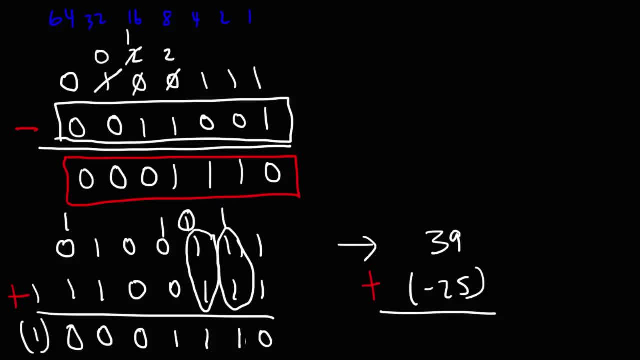 have that many digits to begin with. So now let's see what answer we get. So with this extra carryover, you can just get rid of it because that's an overflow That's going to be out of the range. So our real answer is what we see here: ignoring the overflow. 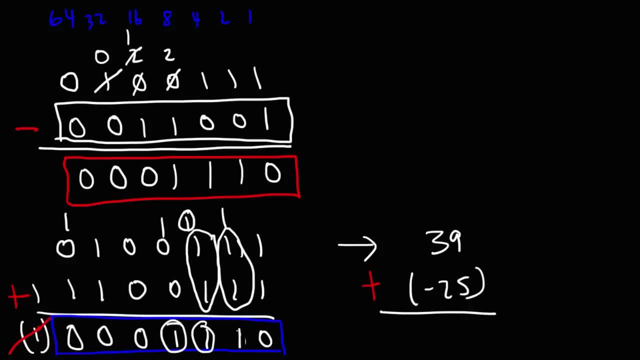 value, And you can see this- is 8 plus 4 plus 2.. 8 plus 4 plus 2 adds up to 14.. So that's how we can do binary subtraction using the 2's complement. So what you want to do is: 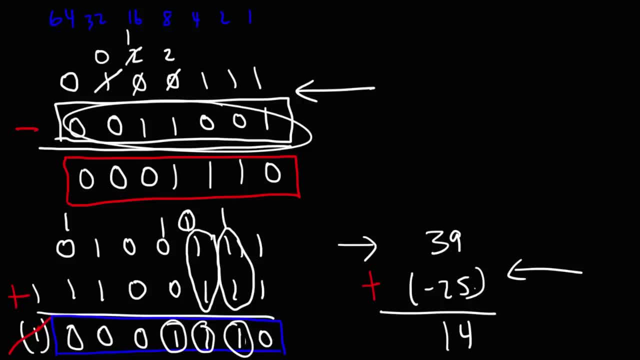 instead of subtracting a positive number, you make that a negative number and then just add it. But you have to get both of these numbers in binary form So you can keep this number the same, but you got to find the 2's complement of this number, which takes a lot of work. 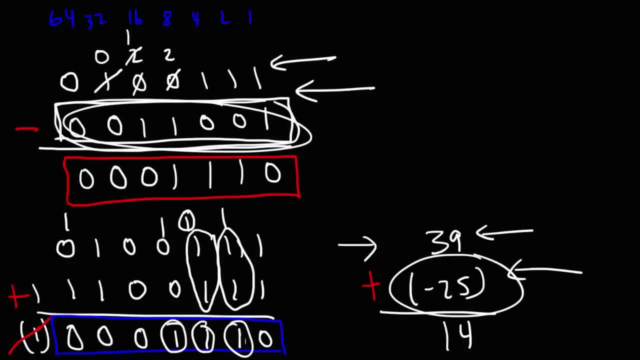 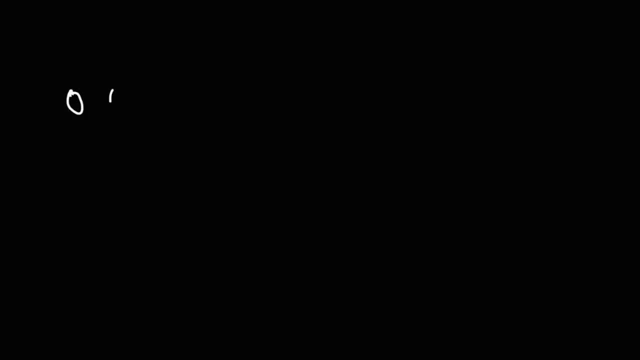 So you have to choose. you know which method is easier for you to do, But that's how you would do it using the 2's complement method. Let's try another example of subtracting two binary numbers. So this is going to be 0, 1.. 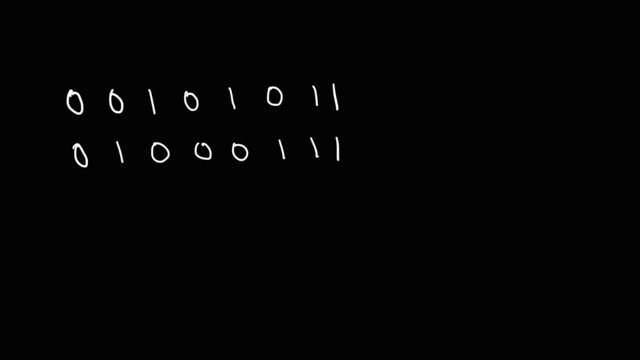 0, 0, 0, 1, 1, 1.. Feel free to try this example Now before I subtract it. I want to get the decimal equivalent of each number. So this is 1, 2,, 4,, 8,, 16,, 32,, 64,, 128.. So this is. 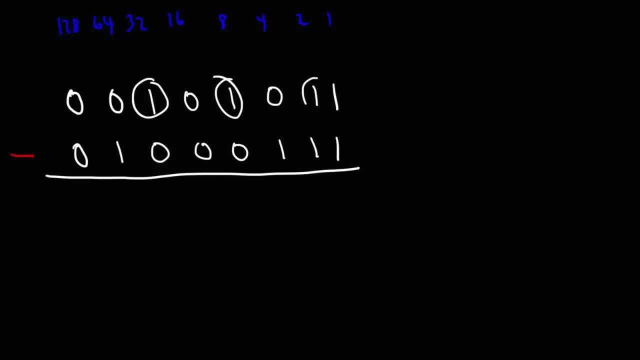 32 plus 8,, that's 40.. 42, 43.. And then we're going to subtract that by this is 64 plus 4,, that's 68, plus 2,, that's 70, 71.. 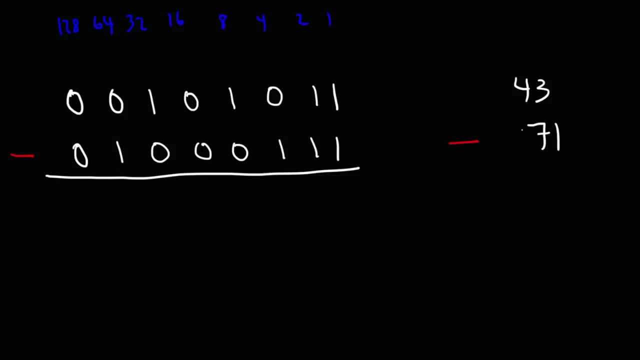 Notice that the second number is larger than the first. Now this is positive 71.. As we can see, the last number is 0. And this is positive 43. So when we subtract these two numbers, we're going to get a negative result: 43 minus 71, that's going to be negative 28.. So will both. 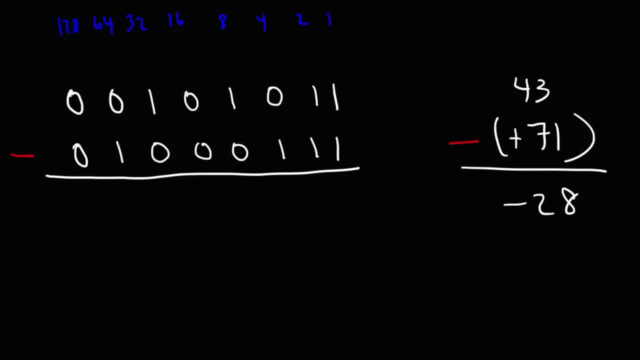 methods give us a negative result. Or should we use the 2's complement method, or should we use the straightforward method? What would you say? It turns out that both methods will work. Let's start with the straightforward method. Let's start with the 2's complement method. Let's start with the 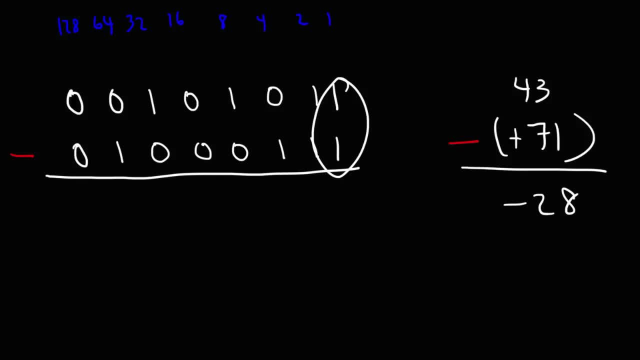 straightforward method. So we have 1 minus 1, which is 0. This is 0 as well. Here we have 1, I mean 0 minus 1.. 0 minus 1 is negative 1.. But you don't want to put a negative number when dealing with. 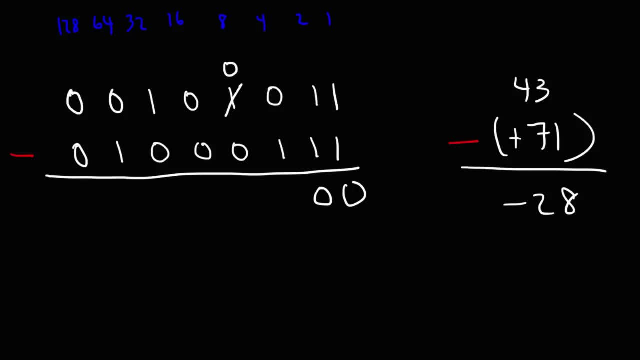 binary, So we'll need to borrow a 1.. This is going to become 2.. 2 minus 1 is 1.. This is 0.. 1 minus 0 is 1.. Now 0 minus 1, we have that situation again. 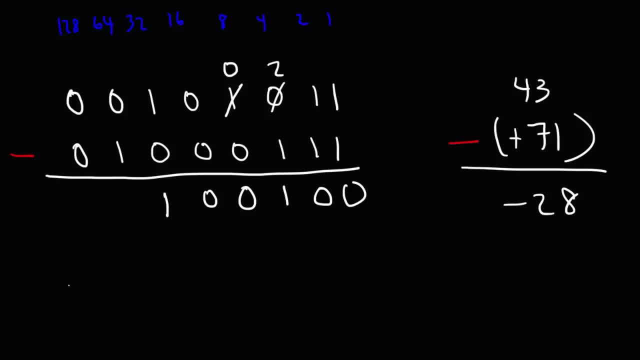 But notice that we can't borrow a 0 here And also it's the last 1.. So in this case I'm going to put negative 1 here, Or rather I'm just going to put 1 in parentheses to indicate. 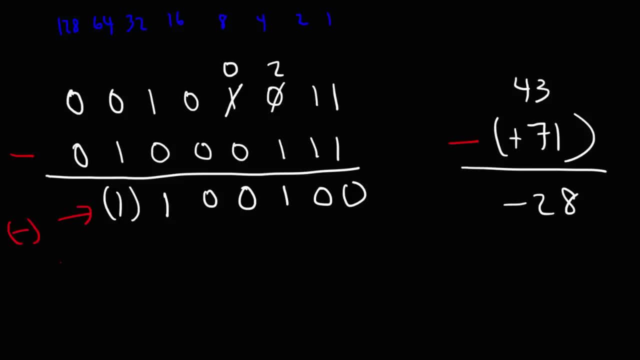 that this is a negative value. Now let's check the work. So we have 64, but this corresponds to a negative value. So that's going to be negative 64. And keep in mind, if the first number is a 1,. 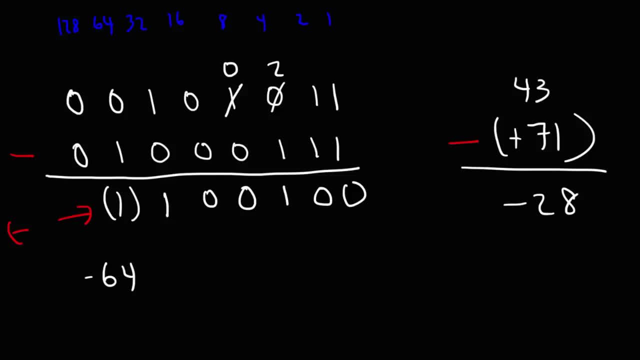 it's a negative value. If it's a 0,, it indicates a positive value. Next, we have 32.. This one corresponds to 4.. And then let's add what we have here. So negative 64 plus 32 plus 4.. 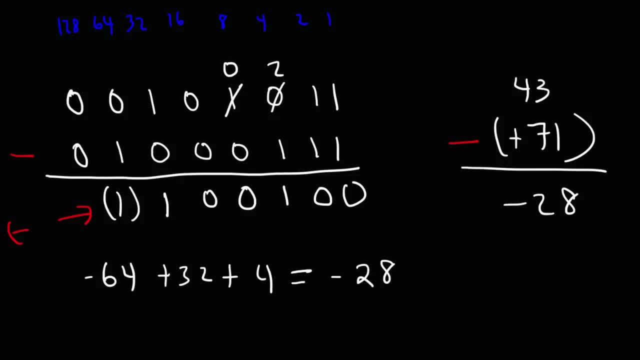 So this adds up to negative 28.. So, as we can see, it does work. So I'm just going to write the answer on the bottom. So this is negative 28 as a binary number. Just keep in mind the first number, 1, corresponds to a negative. 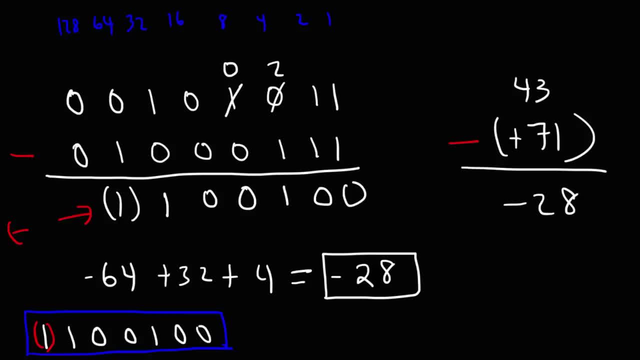 value. Now let's see if we can get the same answer using the 2's complement method. So we are going to, instead of subtracting, we're going to add, But this is going to be negative 71 as opposed to positive 71. And this should give us the same result: negative 28.. 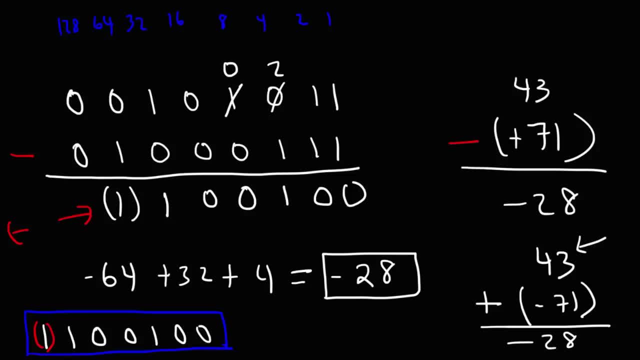 So the first number, 43, we're going to keep the same, But we need to find the negative equivalent of this number. So let's get rid of this. Let's rewrite the top number: 0, 0, 1, 0, 1, 0, 1, 1.. 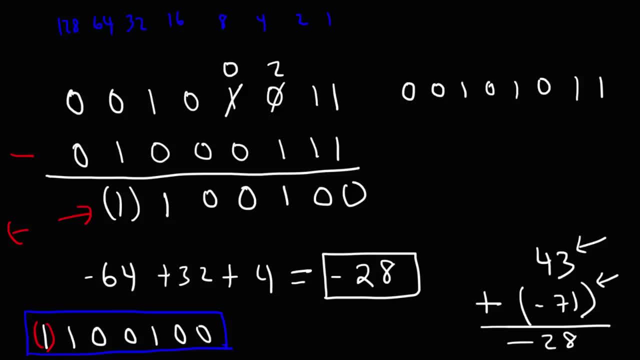 I just had to make sure I copied that correctly. So now let's change this value, And I'm running out of space So I'm going to rewrite it here. Let's find the complement of all the numbers, So let's replace 1 with 0 and 0 with 1.. 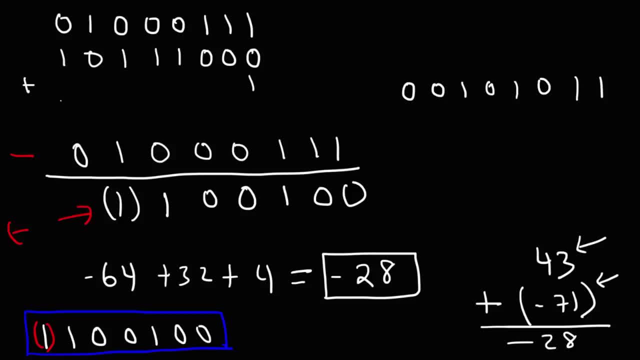 And then we're going to add 1.. So this is going to be 1, 0, 0, 1, 1, 1, 0, 1.. So this should be negative 71. And let's just do a quick check to make sure that's the case. 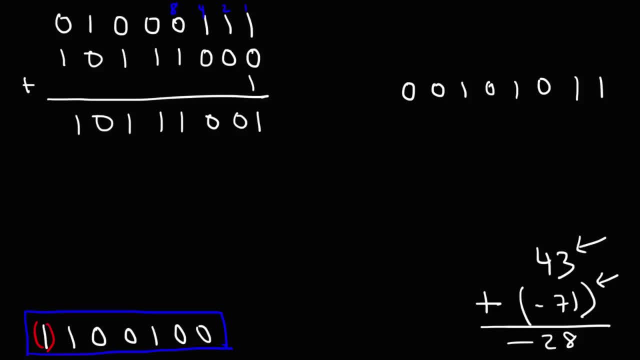 So this is 1,, 2,, 4,, 8,, 16,, 32,, 64,, 128.. Now the first number is negative, So that corresponds to negative 128.. And then we have a 32,, a 16.. 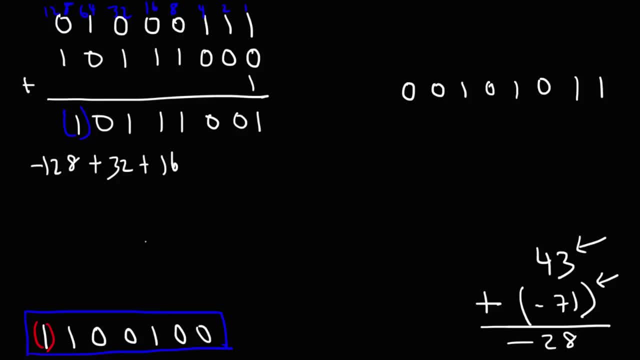 This one corresponds to 8. And the last one corresponds to 1.. So negative 128 plus 32 plus 16 plus 8 plus 1. That adds up to negative 71. So that's the right number. We're going to put that here. 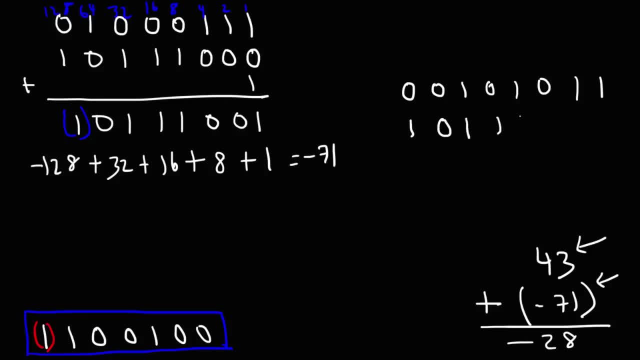 So 1, 0, 1, 1, 1.. 0, 0, 1.. And now let's add these two numbers using this process. So 1 plus 1, that's going to be 0, carry over the 1.. 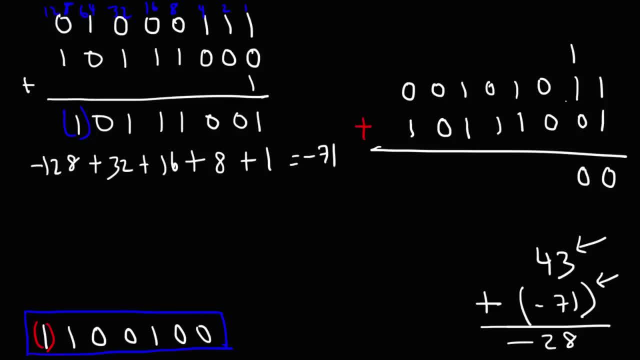 And then we have 1 plus 1 again, which is 0, carry over the 1.. 1 plus 0 is 1.. And then 1 plus 1 is 0, carry over the 1.. Then we have 1 plus 1 again, which is another 0, carry over the 1.. 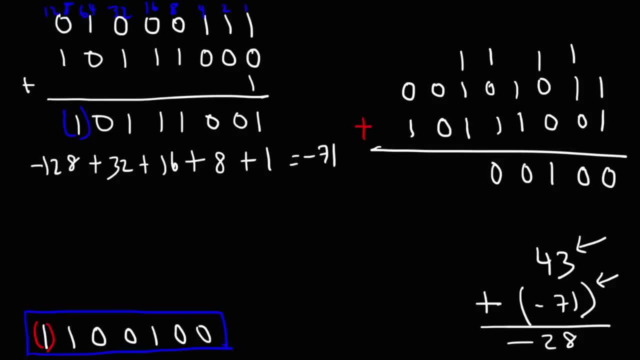 Now we have three 1s, So the first two 1s will give us a 0 and a 1.. And then remaining 1 plus a 0 will give us a 1.. So let's turn that into a 1.. 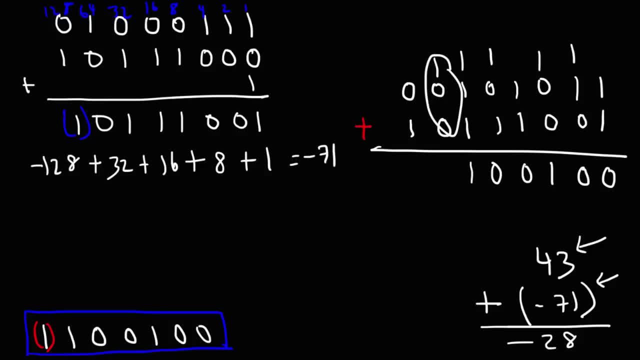 And then we have 1 plus 0,, which is 1.. And then 0 plus 1,, which is 1.. Now our answer looks similar, but not exactly the same. So this part here is exactly what we see here. 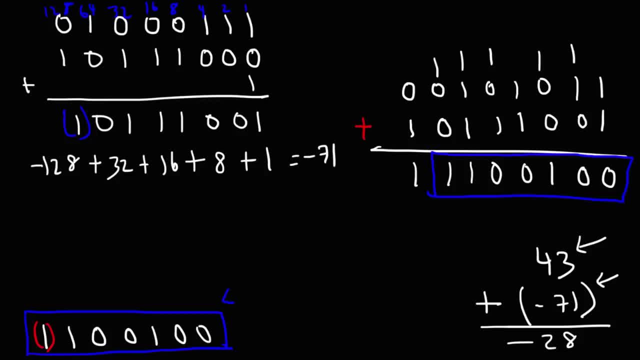 1, 1, 0, 0.. 1, 0, 0. But we got this extra 1.. So why is it different? Well, keep in mind that this is going to be our negative value. It turns out that, even though we have an extra digit, so to speak, or an extra bit, 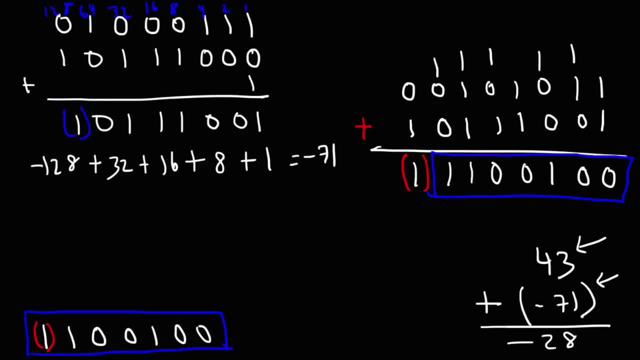 the value is still the same. So this is 1,, 2,, 4,, 8,, 16,, 32,, 64,, 128.. So this corresponds to negative 128.. And then we have a 1 in the 64 column.